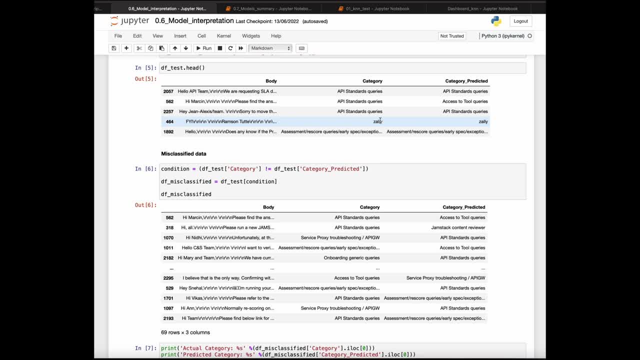 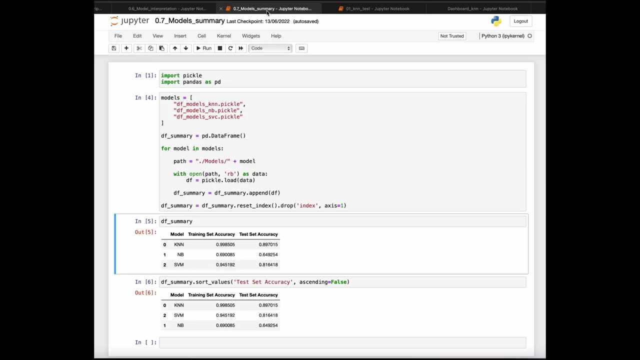 where the actual category and the predicted category do not match. Now this exercise actually helps to analyze the misclassified data and we can see if there is scope of improvement. Now we will see the model summary and choose the best ML model for our example. So I'm 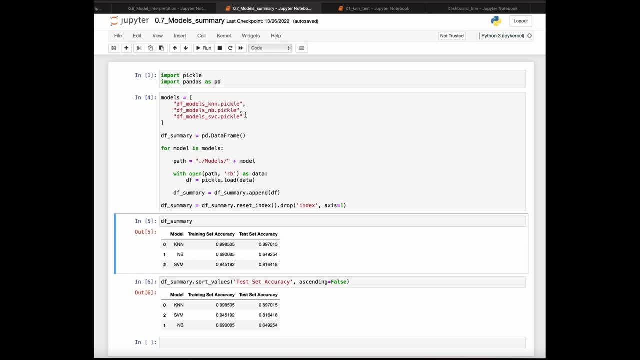 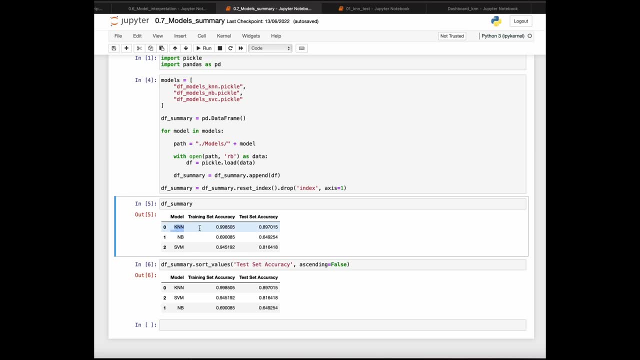 loading all the DF models which I have built in the previous videos And then we are going to see the DF summary here. So, if you can see, here KNN has a test accuracy of 0.89, which is actually 89%. NB naive base has a test accuracy of 64%. 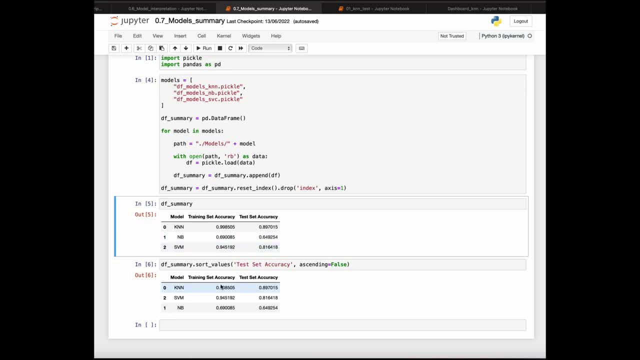 and SVM 81%. Now sorting them according to the test set accuracy, you can see here: KNN tops the chart with 89%, then SVM 81% and then NB. If you can see, here I have loaded our KNN model. 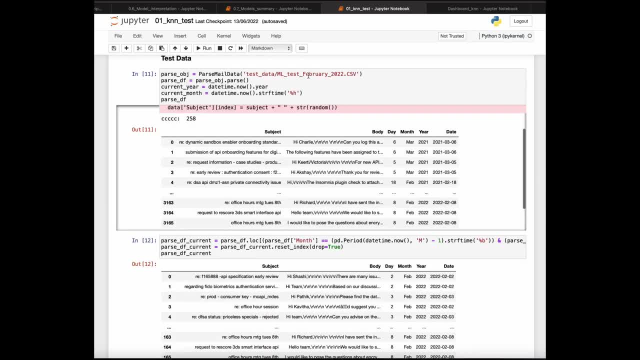 And then I'm going to fit the test data into our model to actually predict the categories. Now the test data. if you see, here one of the modifications which I did is adding the day, month, year and date in the data frame. 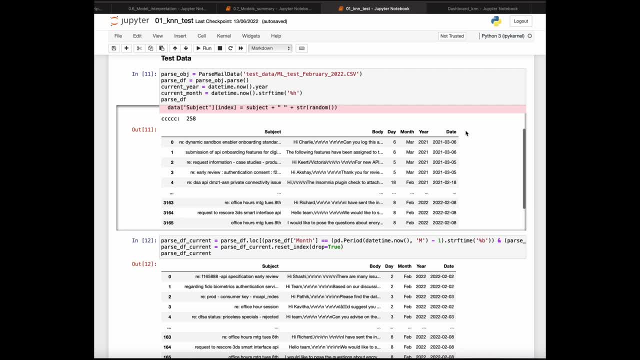 This was actually our use case because we have to analyze the data month-wise. So I wrote a parser which actually reads the body of the email and then fetch the date, And then I've used it to populate the state. Now I'm going to use this test data to predict the categories, Like if you see here I have 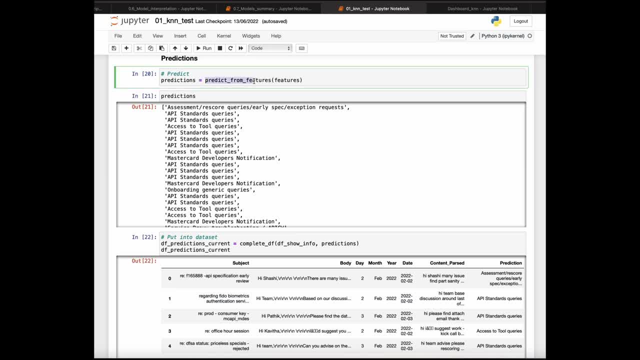 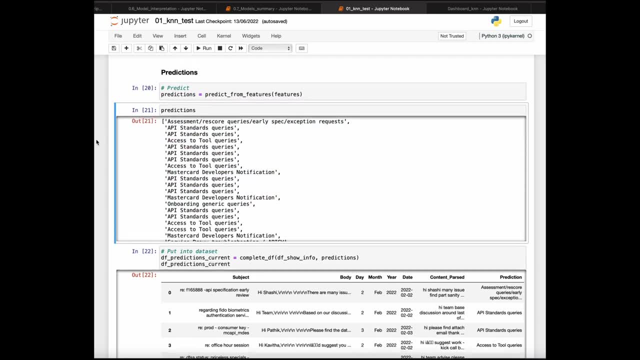 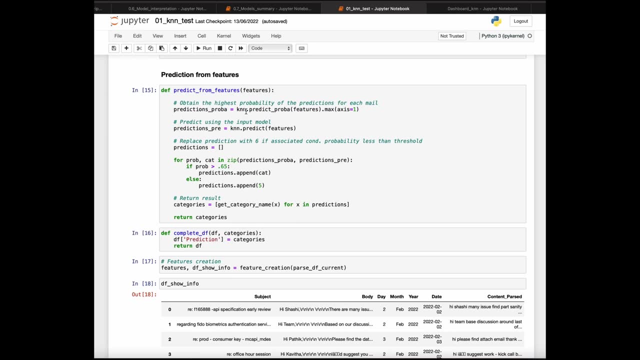 created one function called predict from features, and then I have used the features to actually predict the categories, And these are the categories which are predicted for the test data. If you see the predict from features function, this is actually the same thing. I have used the KNN model which we had built before, and then I'm going to predict the 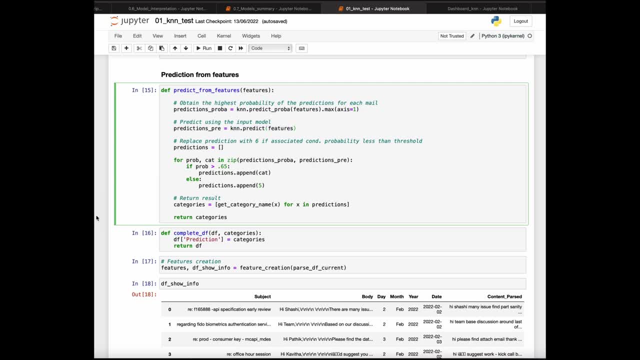 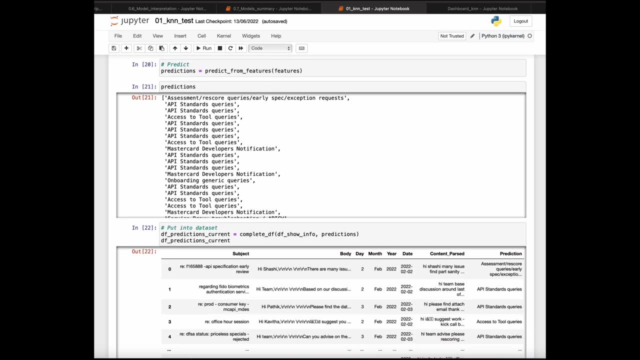 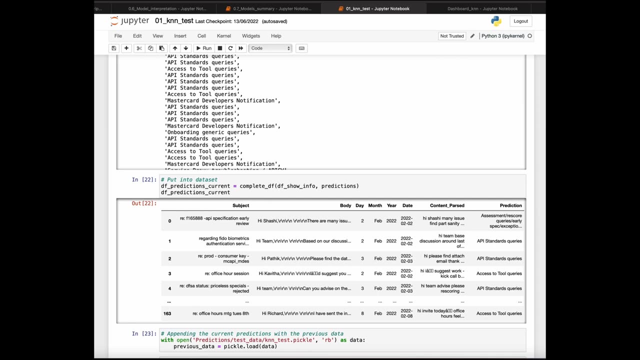 categories here. Now I'm going to add the category column in the data frame and save it as a pickle file so that I can use that later for visualization of the data In the next video. we are going to use this data frame and visualize our data through. 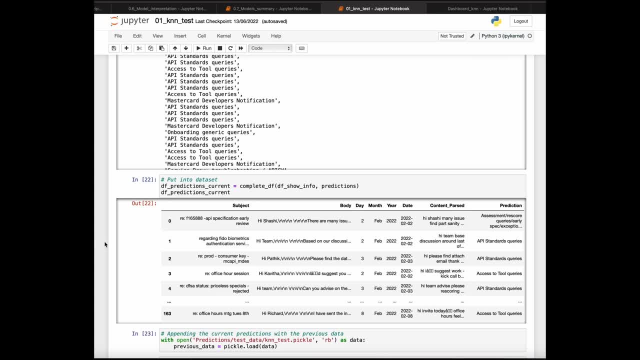 graphs. I've also built an app to visualize the data through graphs. We will see that in the next video.